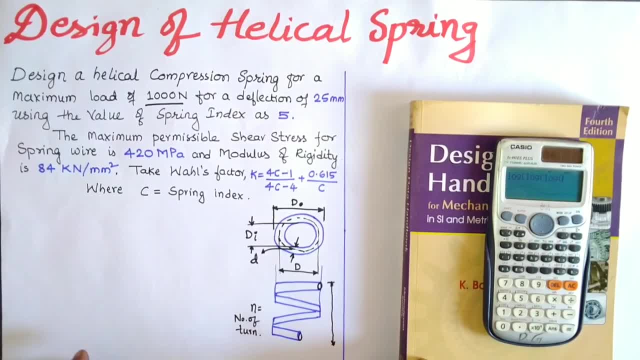 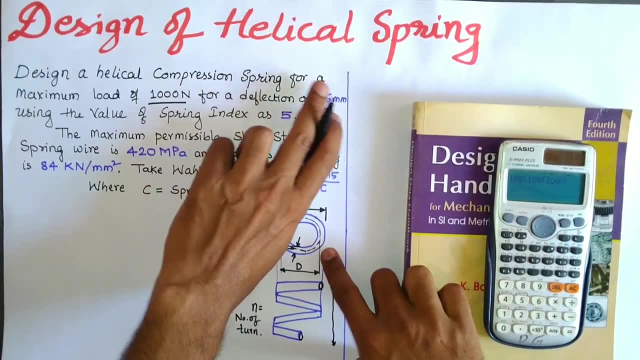 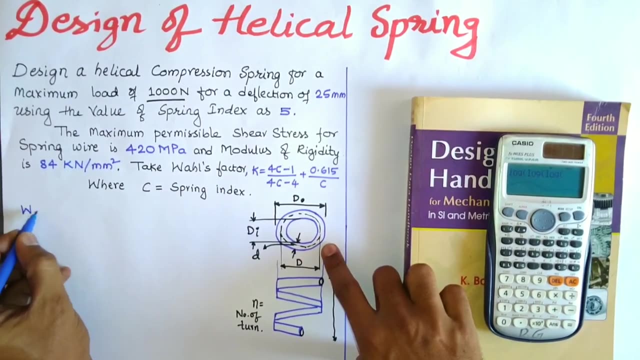 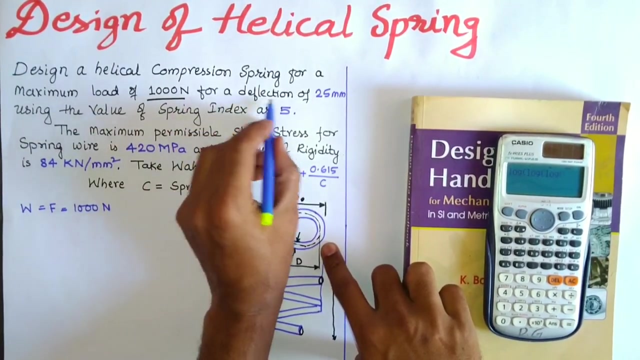 Okay, so after that we will read the question. design a helical compression spring for a maximum load of 1000 newton, So where the load will denote with w, or you can write f, as 1000 newton for a deflection of 25 millimeter. 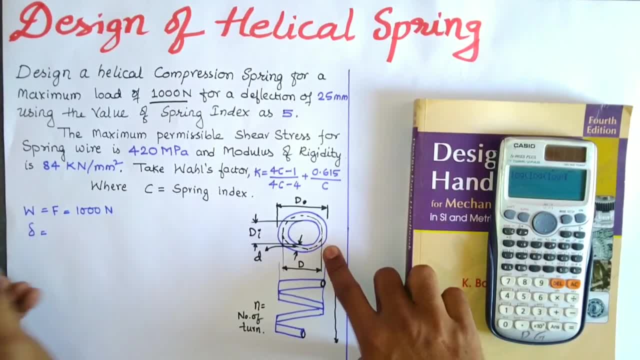 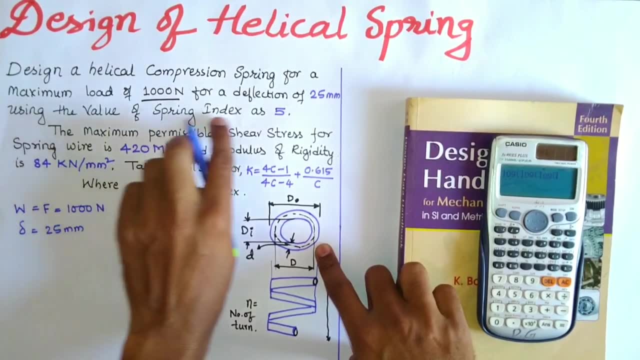 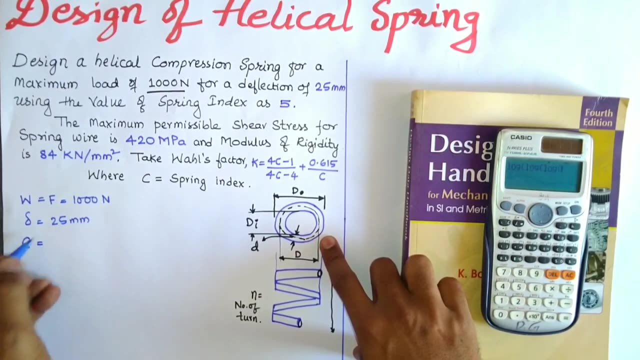 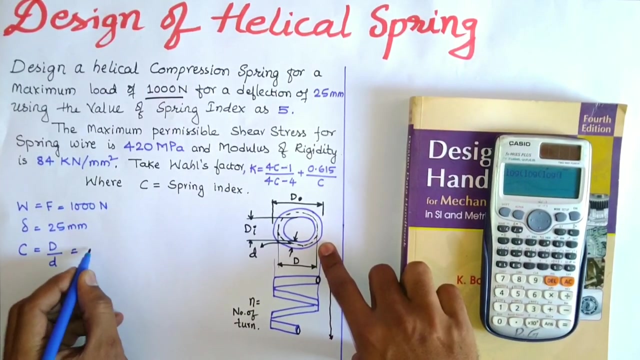 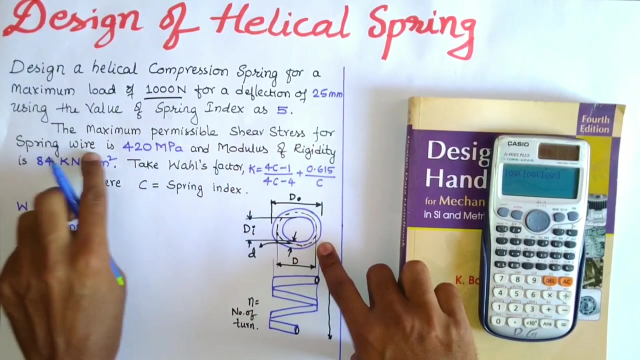 So deflection, that is delta we will present, is equal to 25 millimeter, using the value of spring index as five. So spring index it will be denote with c. So spring index is the ratio of outer diameter by inner diameter. So that value is five is given and the maximum permissible shear stress for this spring wire is 420. 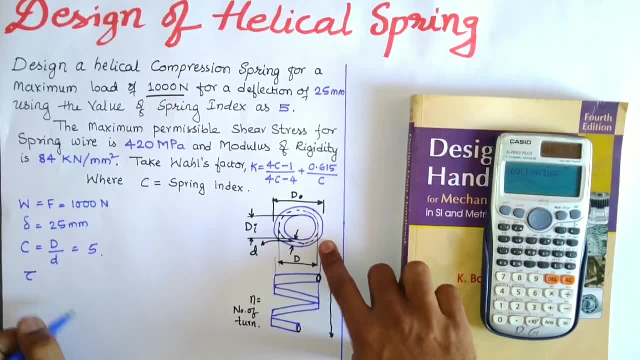 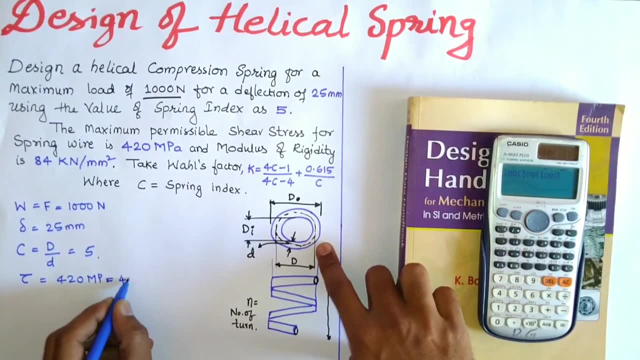 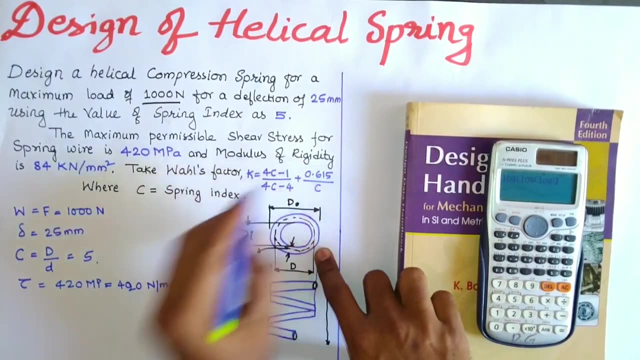 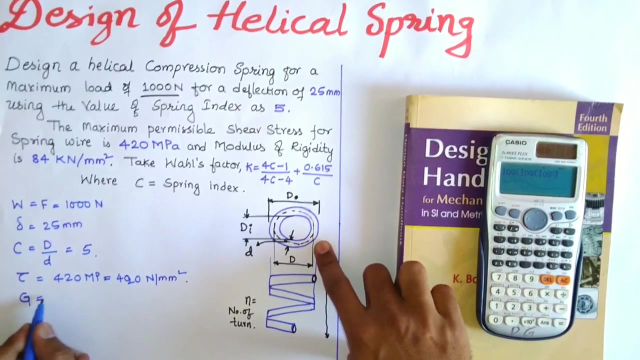 Megapascal. so shear stress is, as tau is equal to 420 mega pascal, So 420 newton per millimeter square, and the modulus of rigidity. So modulus of rigidity, it will be denoted by g or some textbook, it will be denoted by c. 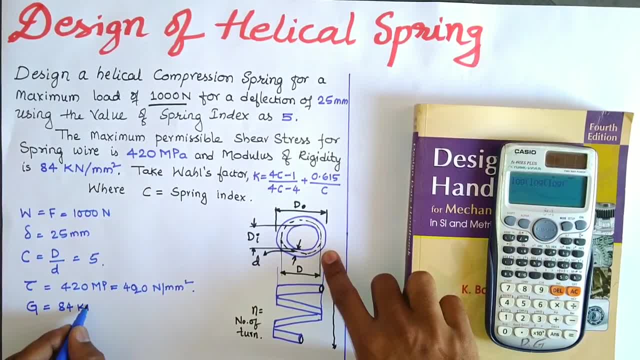 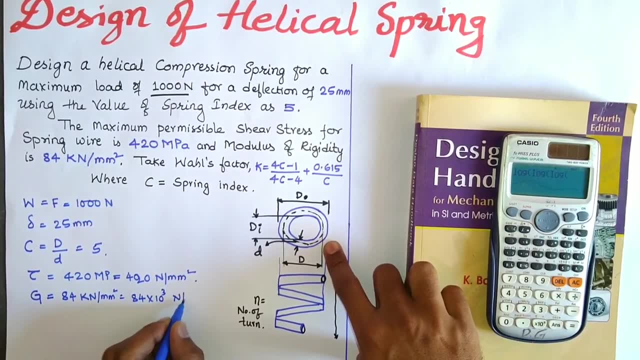 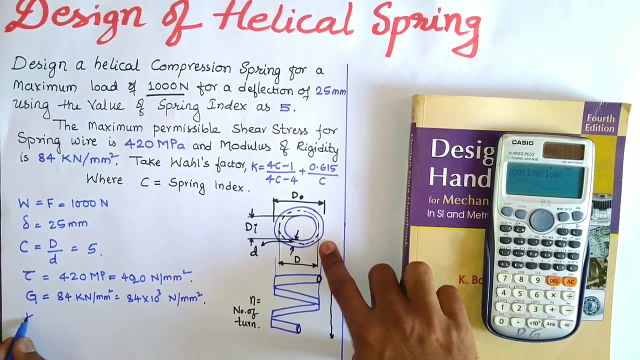 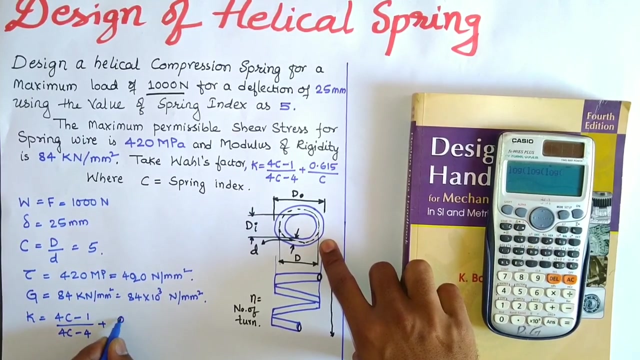 So that value is given as 84 kilo Negotiations Newton per millimeter square. So 84 into 10 power of 3 Newton per millimeter square. and take walls: factor k is equal to 4c minus 1 divided by 4c minus 4 plus 0.615 by c. So 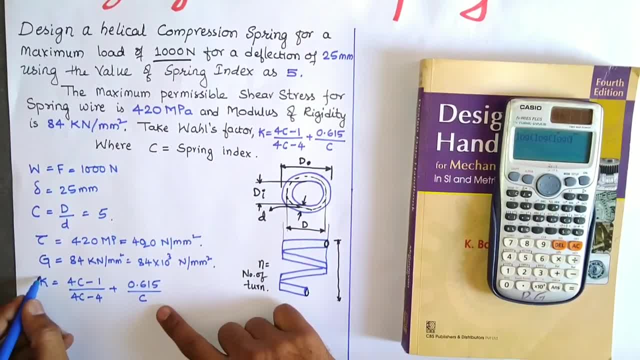 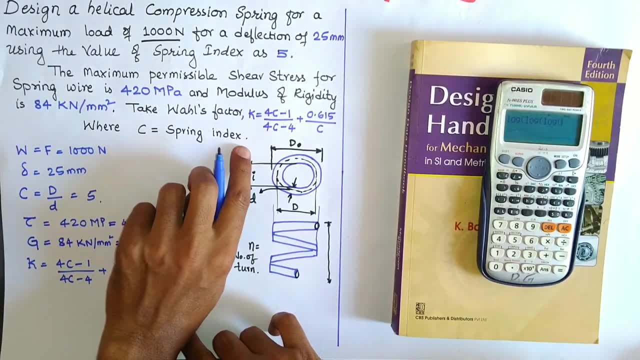 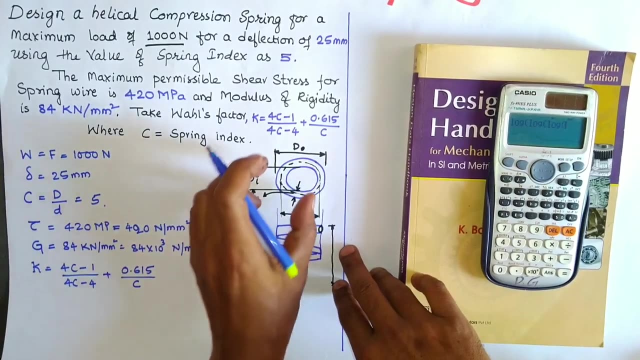 this k value is already mentioned in the question. If it is not mentioned also, we can take from the design data handbook, where here c is the spring index. So now, first thing: while designing the helical compression spring, the main factors, main parameters are to calculate the first thing. 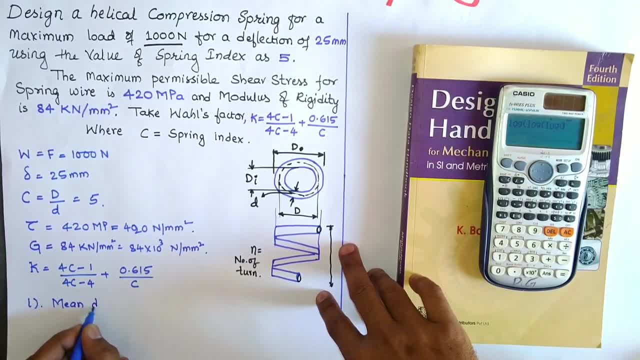 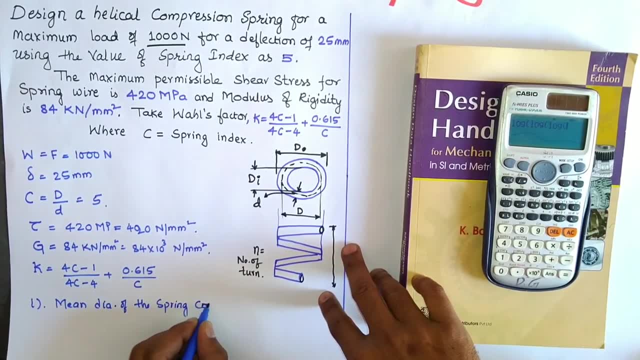 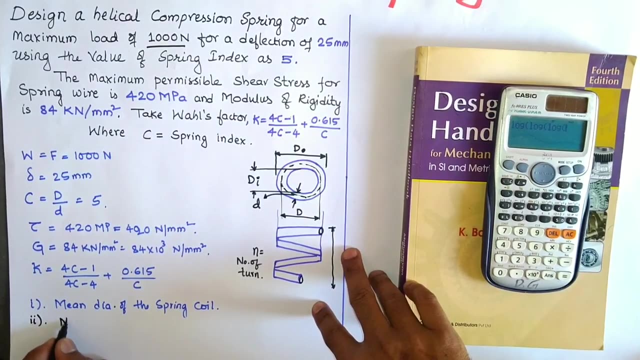 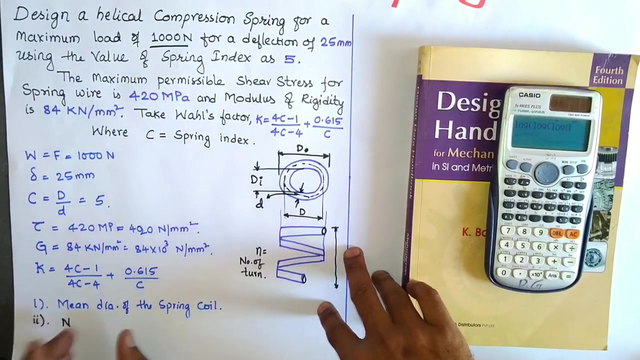 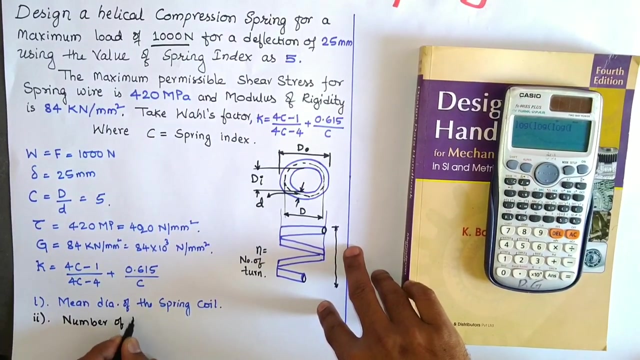 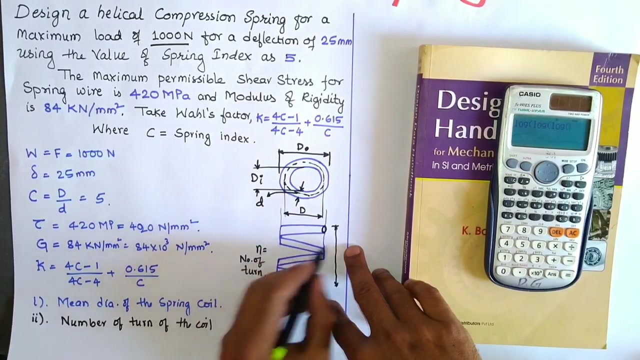 to calculate the mean diameter. mean diameter of this spring coil. And the second one is to calculate the mean diameter- means it will be outer diameter, inner diameter and the mean diameter, all the diameter you have to calculate in the first step. Second, the number of turns. number of turns of the coil, So n number of turns. 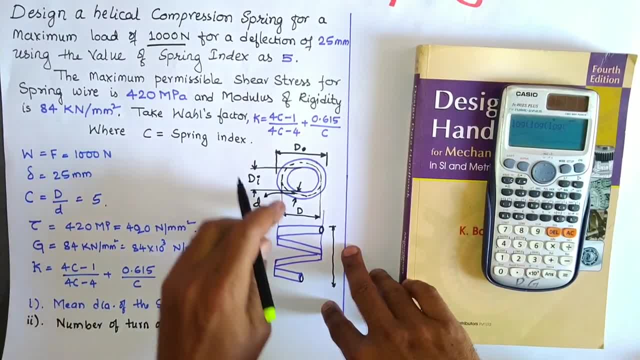 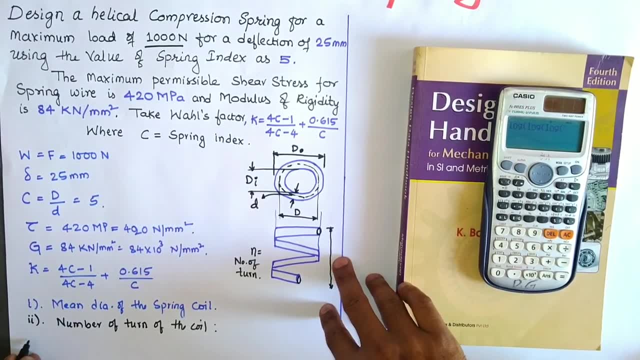 in the coil and in this you are going to calculate the total length of the coil and when it is free to expand. that also you need to calculate. in the second step and in the third stage you are going to calculate the free length. that's only I. 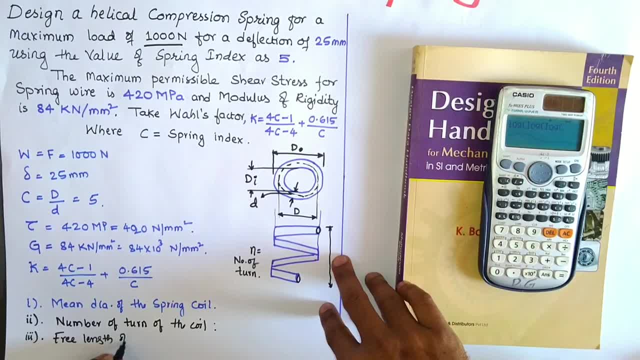 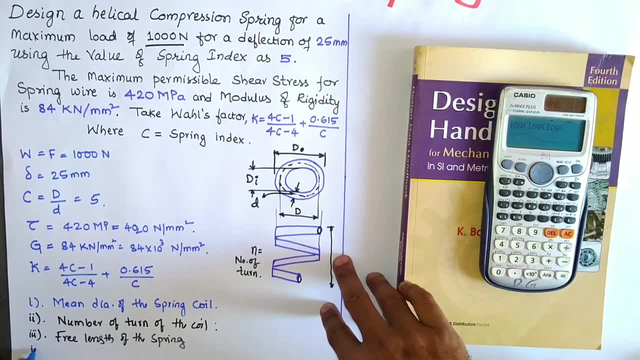 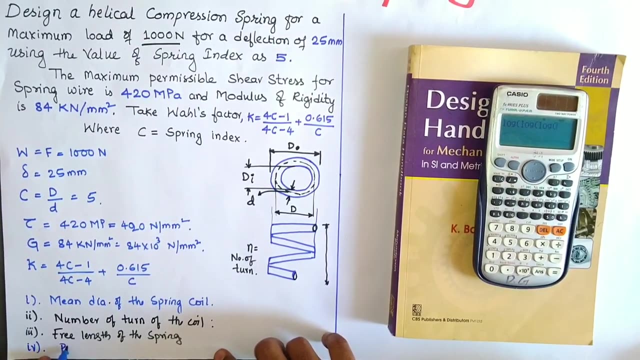 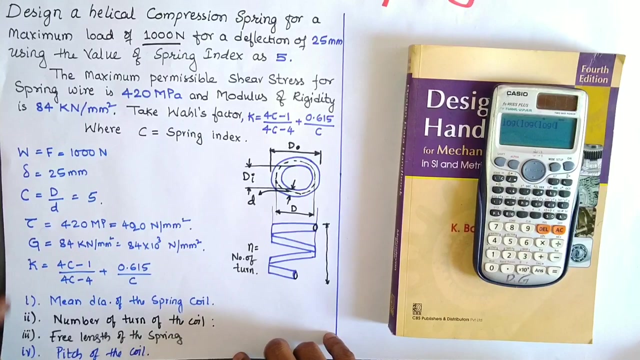 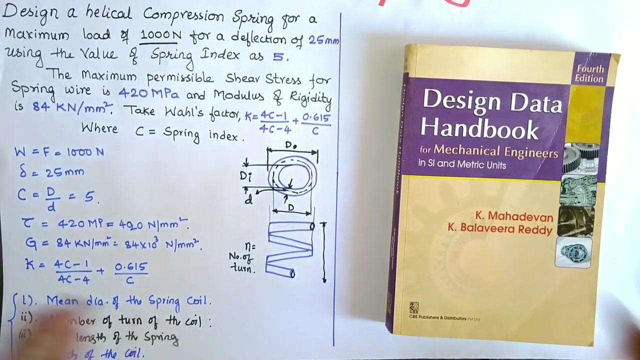 told no free length of the spring. when it expands, what will be the length of the coil you have to calculate. then, lastly, you need to calculate the pitch of the coil. pitch of the coil you have to calculate. so in in the design, it consider these four steps, using you to follow. okay, so here, first thing will: 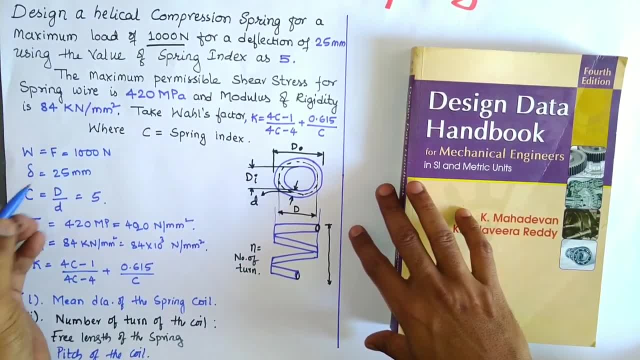 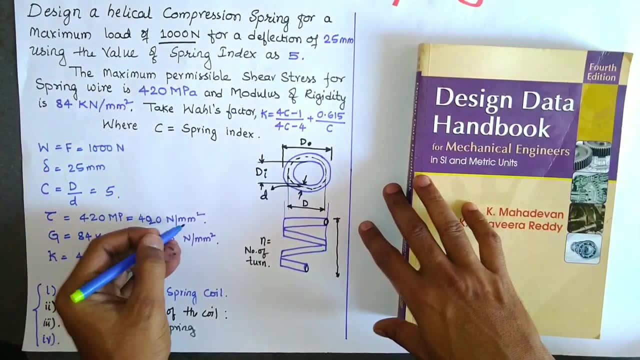 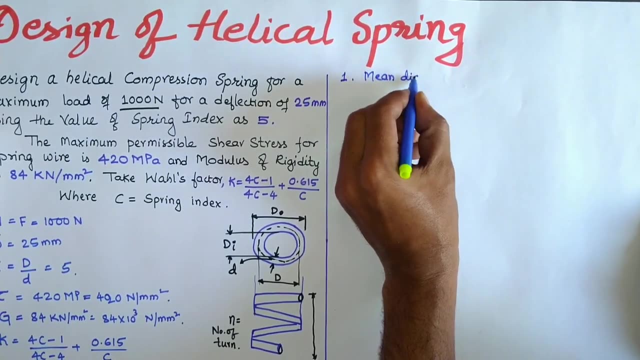 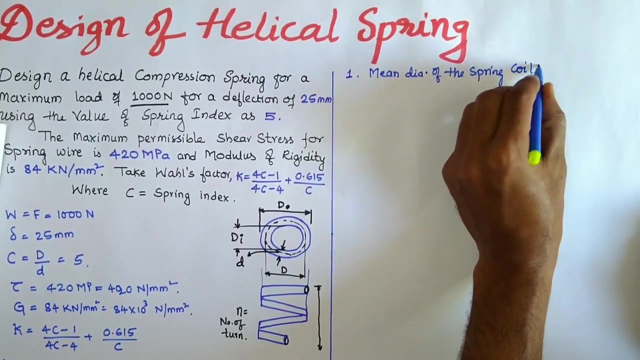 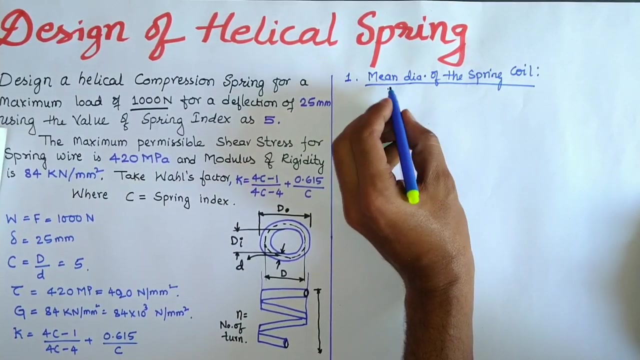 calculate the mean diameter of the coil. so we have, we know that all diameters are in millimeter. here dicen indiscriminمر o of the coild 감�ك. so it will be the mean diameter of the coil. capital D, so it will be the mean. 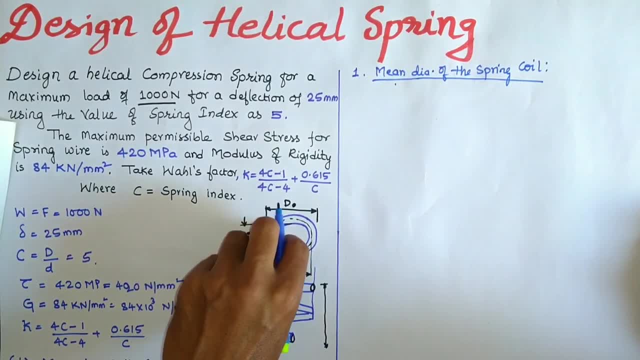 diameter of the coil capital D. so it will be the mean diameter of the coil capital D. So here, first, where capital D will be the mean diameter of the coil capital D, it can friendly andบ and small d, it will be the diameter of the wire. okay, so after that, as we know, 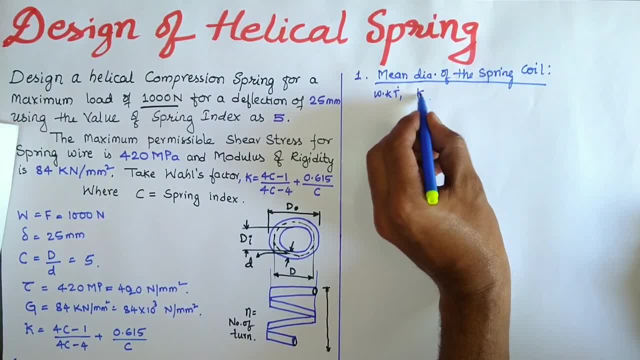 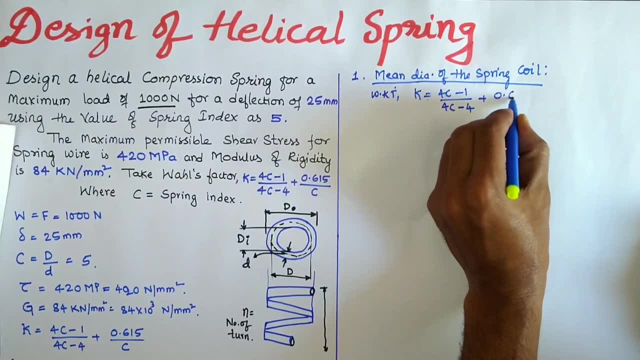 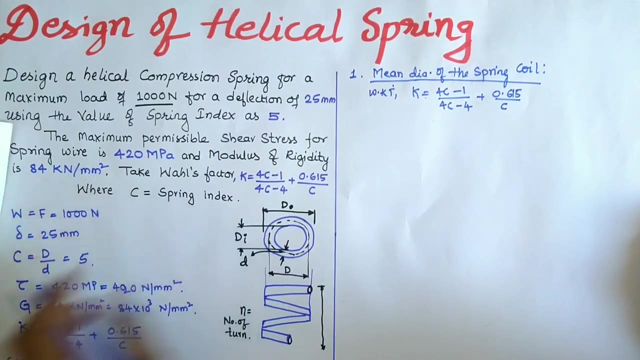 that we know that where K is equal to 4 C minus 1 by 4 C minus 4 plus 0.65, 615 by C. okay, so we will substitute the value of C spring index is given in the question, that is 5. so we can substitute here to calculate the K value Walsh. 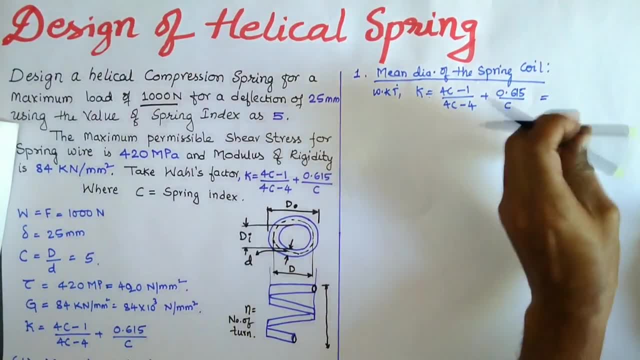 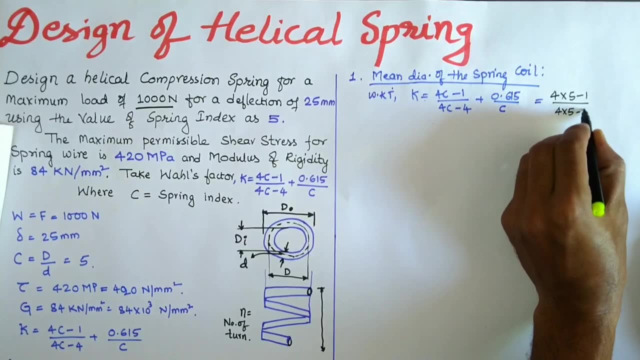 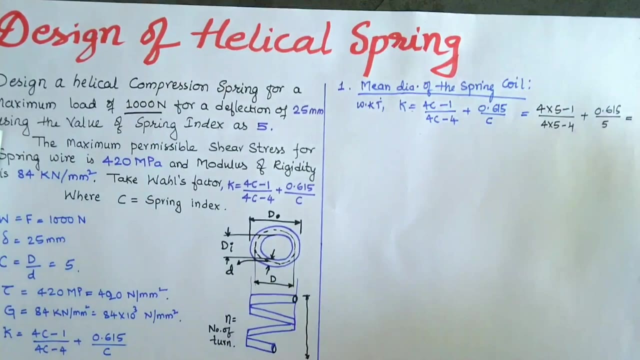 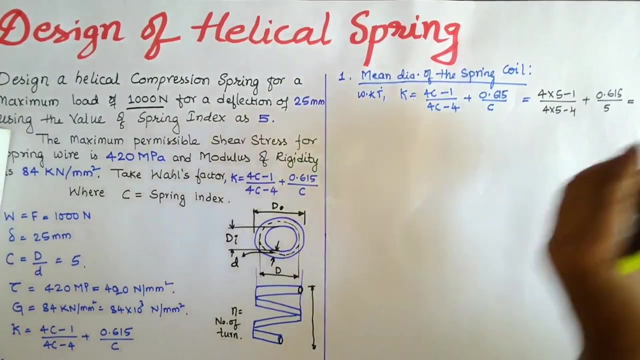 factor. so 4 into C is 5 minus 1 divided by 4, into 5 minus 4 plus 0.615 divided by 5. so here we will calculate the value. so here we will calculate the value. so so here we will calculate the value. so 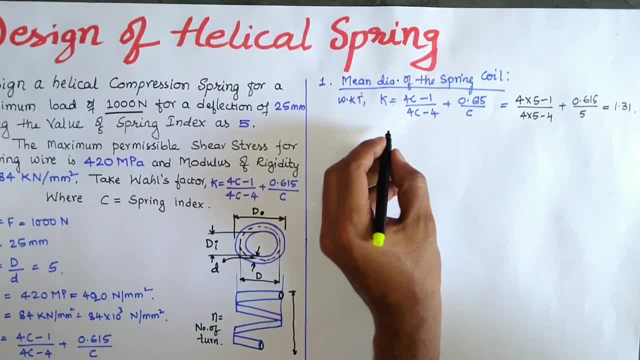 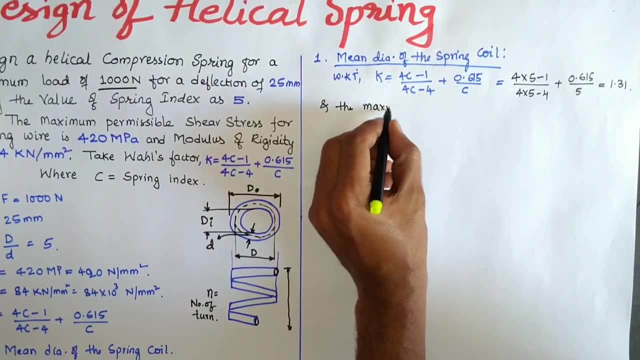 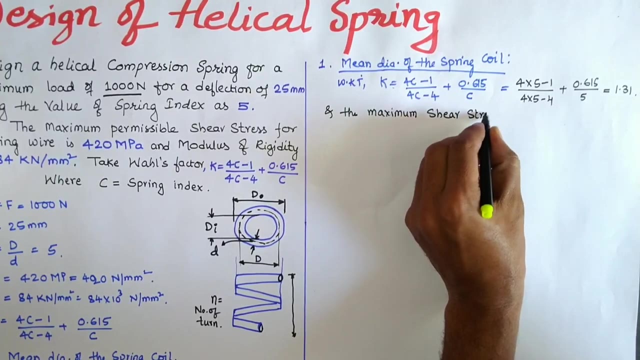 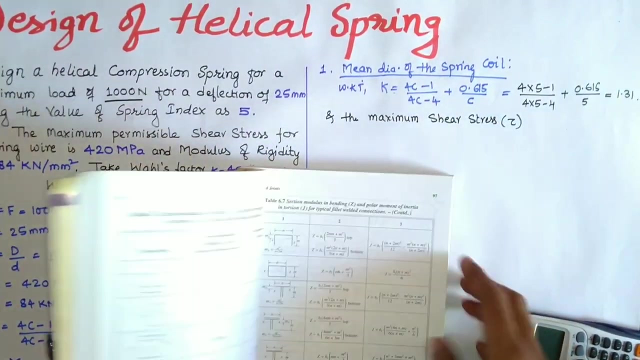 got 1.31, is the K value, okay, and the maximum stress, maximum shear stress, where tau is equal to. so I will tell you how to find this equation in the design data and book. so in page number 167 will have the spring data and book. so in page number 167 will have the spring. 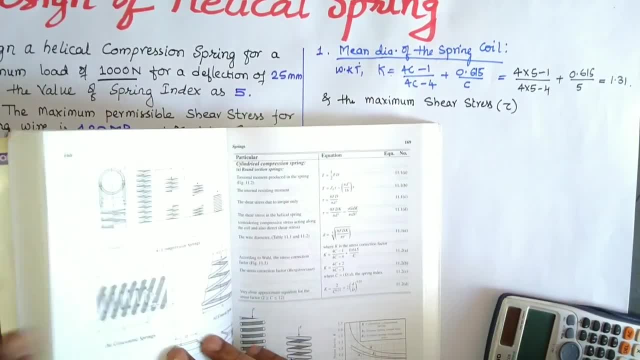 data and book. so in page number 167 will have the spring of springs here. so while in the design of of springs here, so while in the design of of springs here, so while in the design of spring, so it is for the compression spring, so it is for the compression. 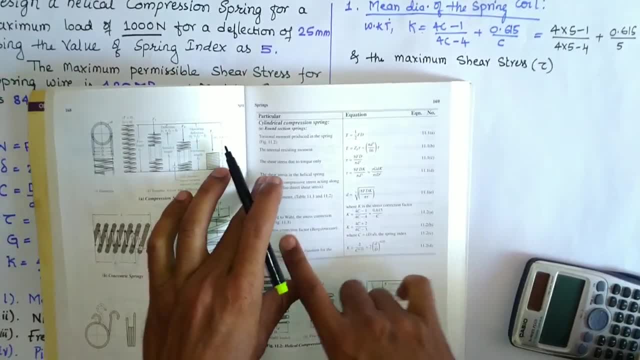 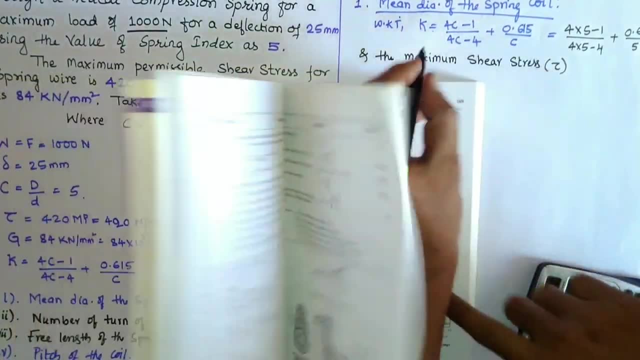 spring. so it is for the compression spring. so here the walls factor is also spring. so here the walls factor is also spring. so here the walls factor is also given according to the walls stress given, according to the walls stress given, according to the walls stress concentration factor in the 11.2. so this: 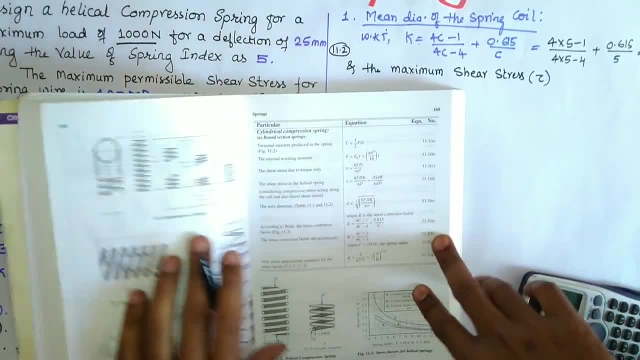 concentration factor in the 11.2. so this concentration factor in the 11.2. so this equation you can find in 11.2. okay, in equation you can find in 11.2. okay, in equation you can find in 11.2. okay, in page number 169. so where the walls 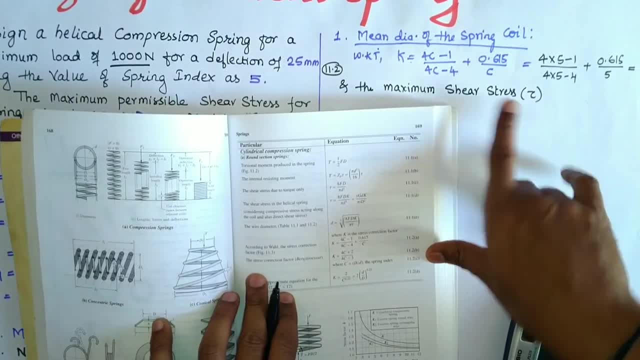 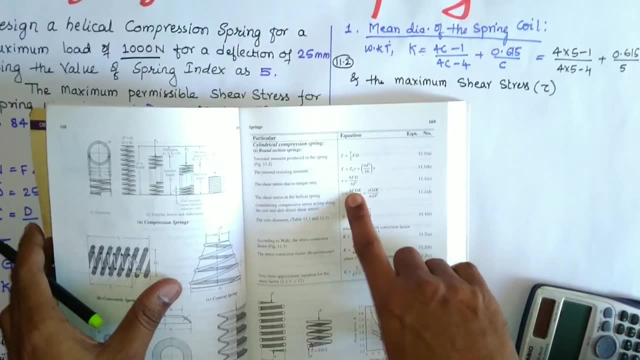 page number 169. so where the walls factor is given after that to calculate the maximum shear stress, that is tau, so shear stress in the helical spring. so the equation number 11.1 d, so tau is equal to 8 fd k divided by pi d cube. 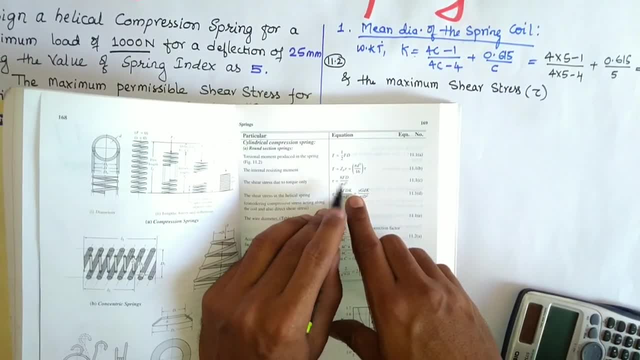 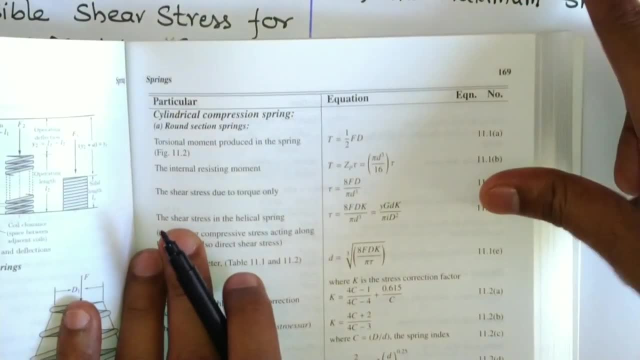 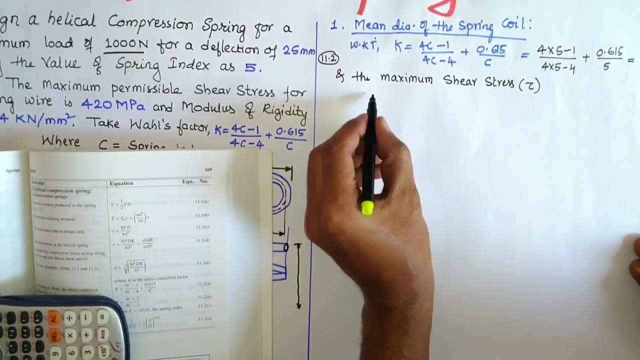 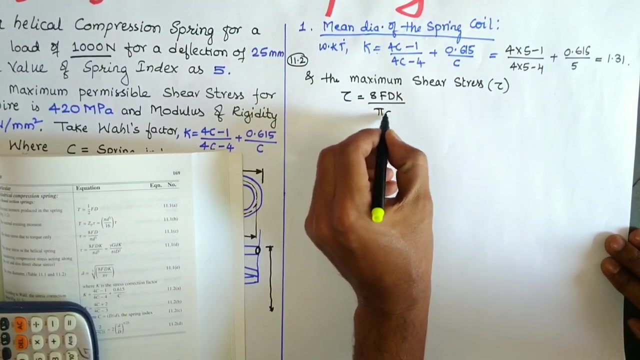 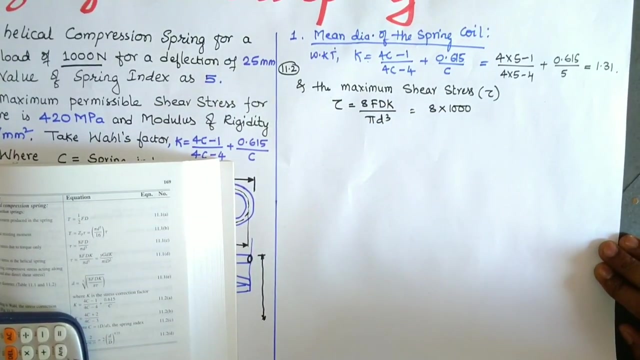 where f it is called as load and d is the mean diameter of the coil and k is the walls factor divided by pi d cube. okay, so to calculate this one, i will write the shear stress where tau is equal to 8, f, d, k divided by pi d cube. okay, 8 into f is 1000, that is load into. 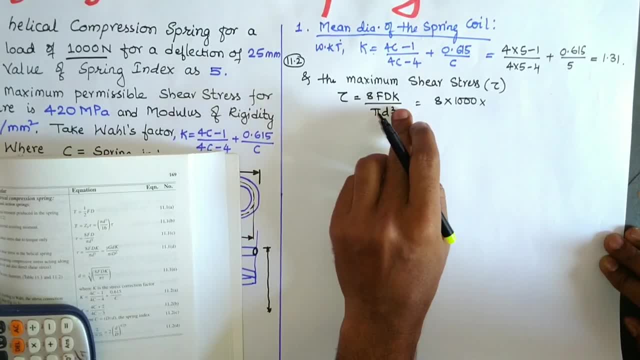 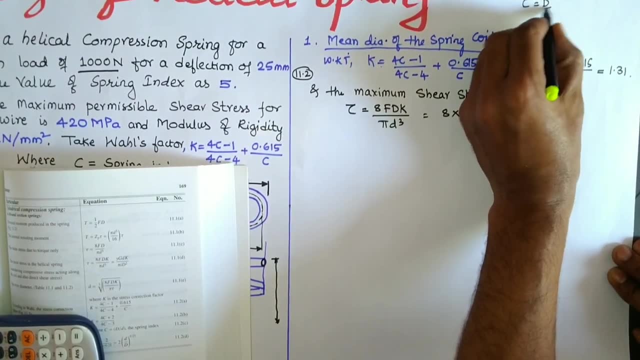 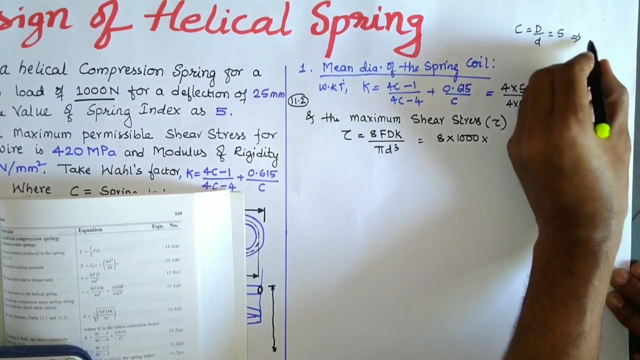 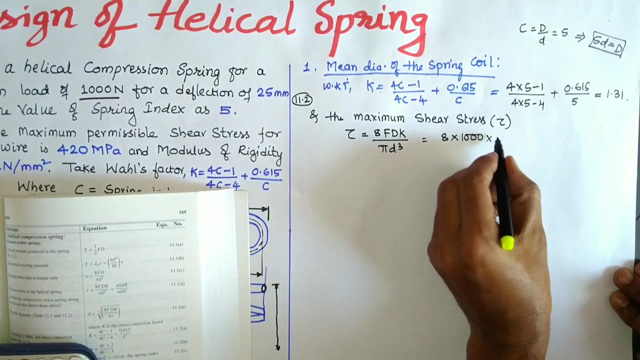 d, so mean diameter. we have not calculated so mean diameter. where c is equal to it is as c is equal to. we have d by d right. so that value is 5. so to calculate d it will be 5 into d. where capital d is equal to 5 into d, we can take from the given value, so 5. 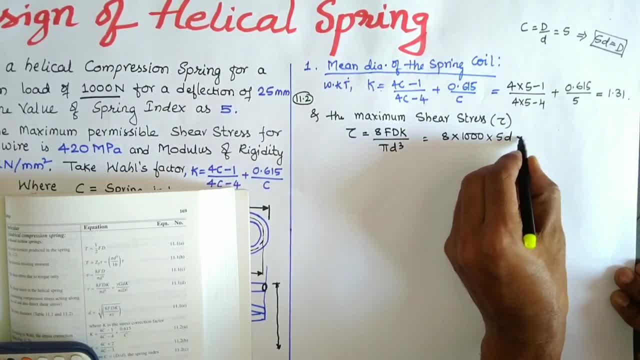 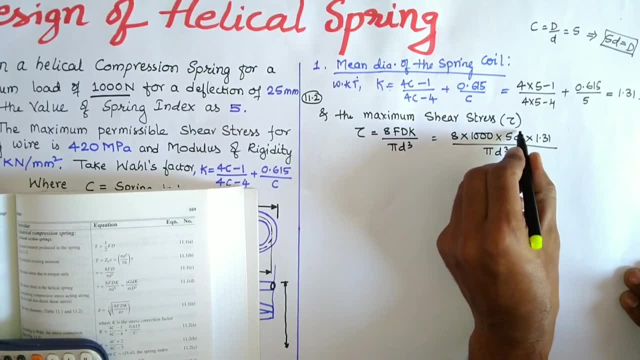 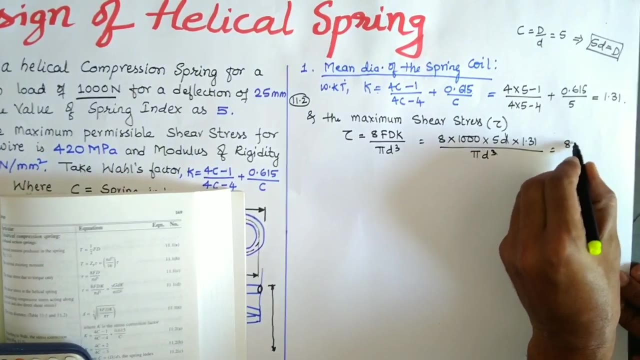 into small d into the k value is 1.31 divided by pi d cube. so here 1 d and this d will get cancelled and 1 on that will be c of nine times d divided by pi 2 жизd square. so here it will be d square. so 8 into 1000 x 5 into 1.31 divided by pi d square. okay. 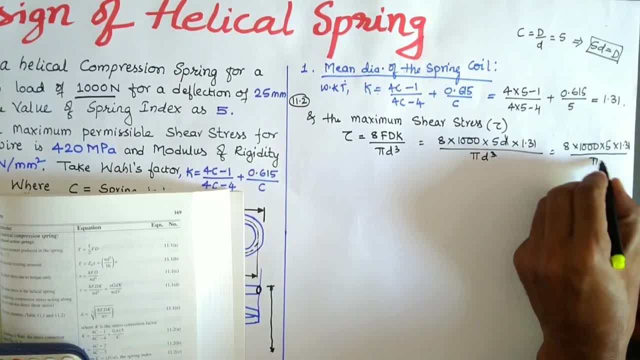 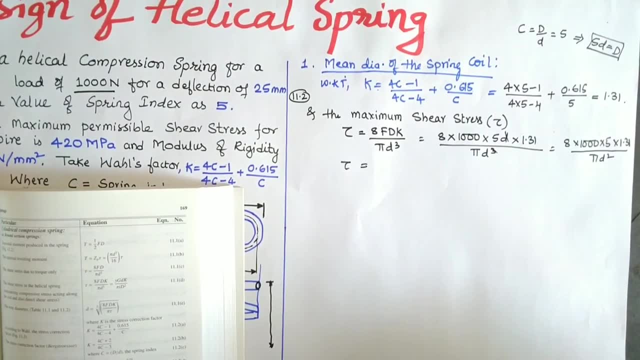 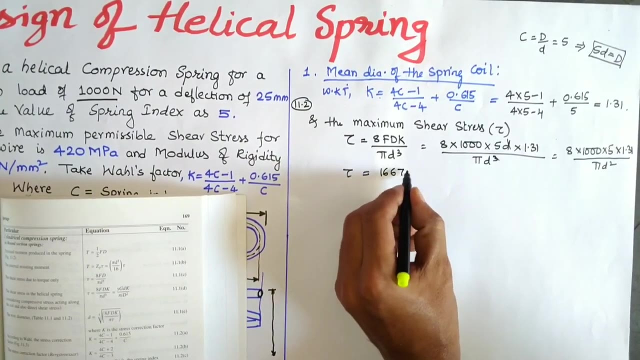 1 on. that will be d squared x 5 into 5 into 1.31, divided by pi d squared. okay, we'll see what the value will get here after making the multiplication, including pi. so we will see one. we will negate k after making the multiplication, so we got this: 16000 677. 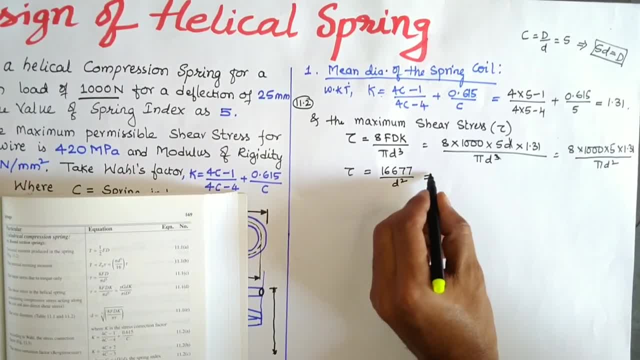 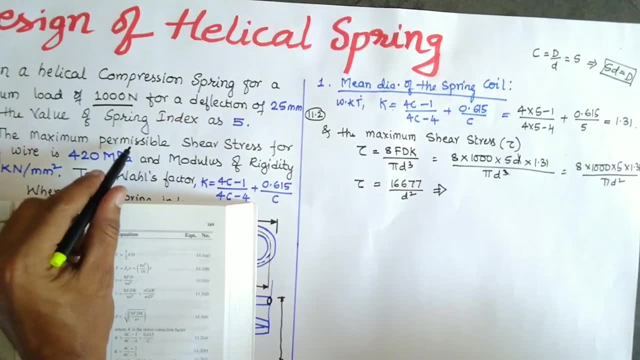 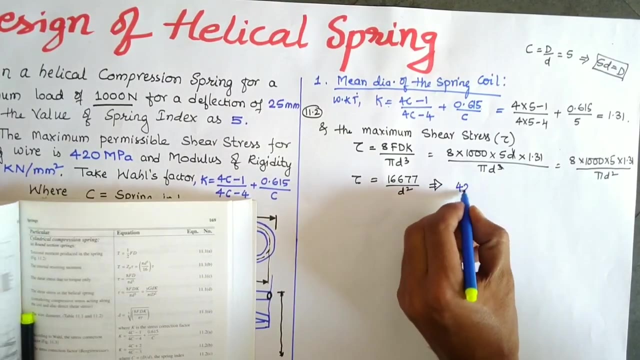 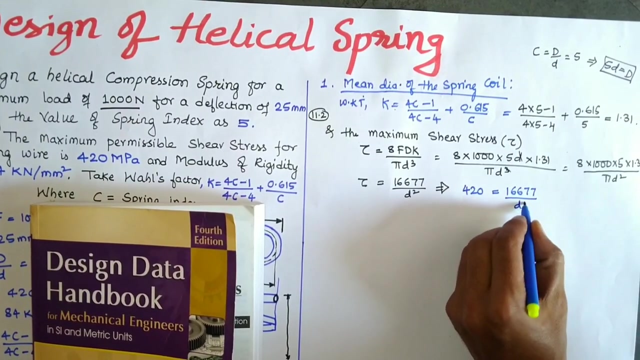 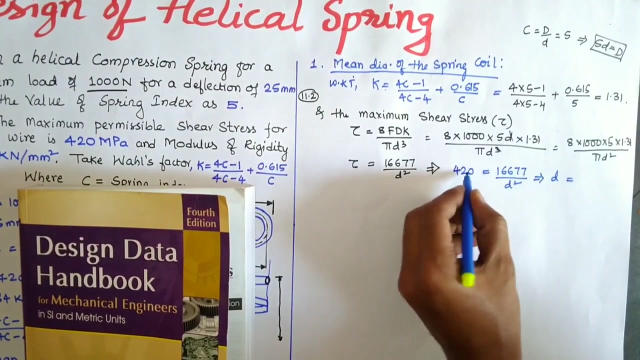 So here the shear stress is mentioned in the question. the maximum permissible shear stress for the spring wire is 420, so we have to substitute the value of 420. as tau is equal to 16677 divided by d square, so is equal to now we will get the value of d, so d square. 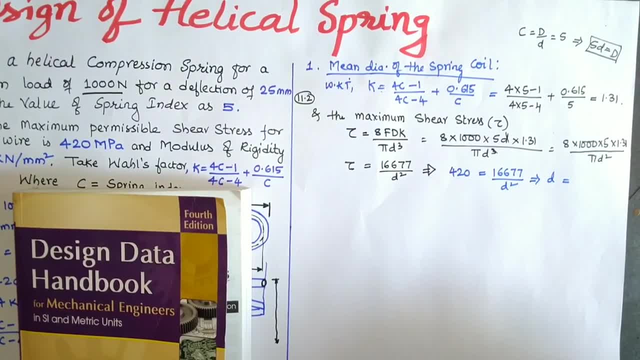 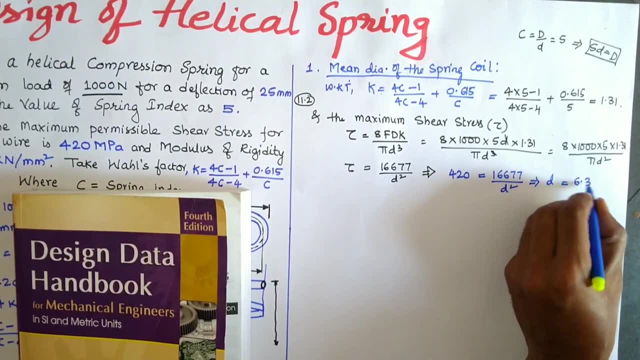 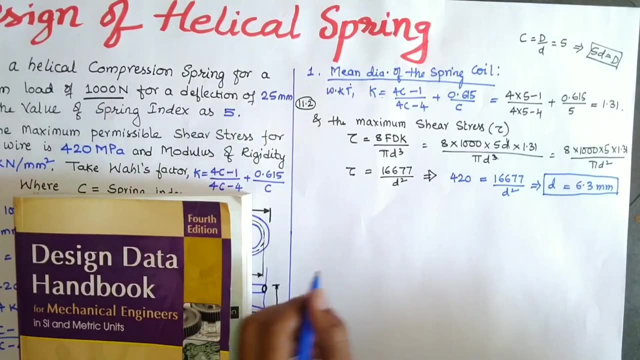 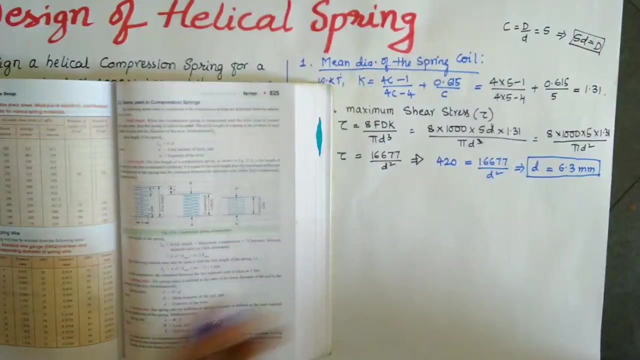 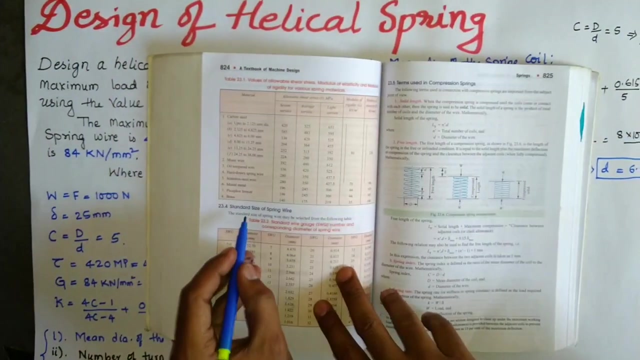 to be changed into d. So now 16677 divided by 420 under root of the answer. so we obtain 6.3 mm is the diameter of the spring wire. So now from the table. so the obtained diameter is 6.3 mm. now to refer the design data handbook. 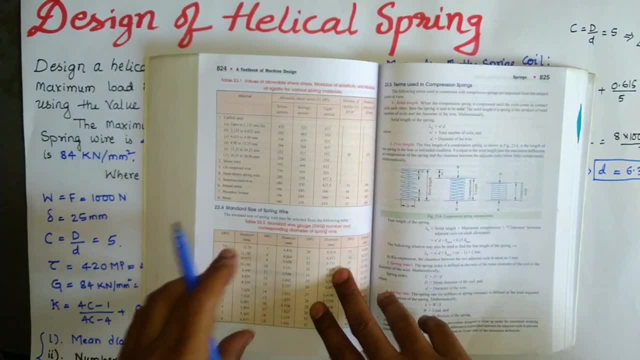 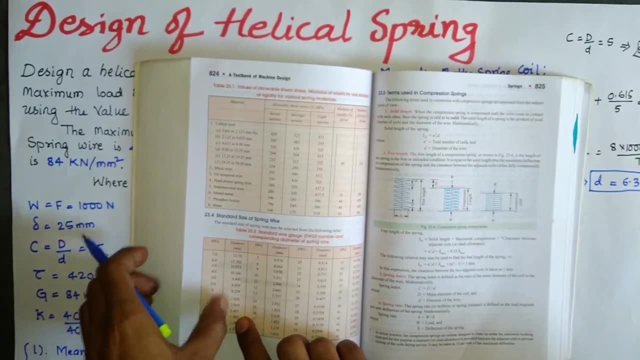 so here are the standard size of the spring wire. so what is the standard size near to the 6.3,. so here, 6.401 is the standard diameter for the wire gauge according to the wire gauge standard wire gauge. So 6.401 is the standard value. 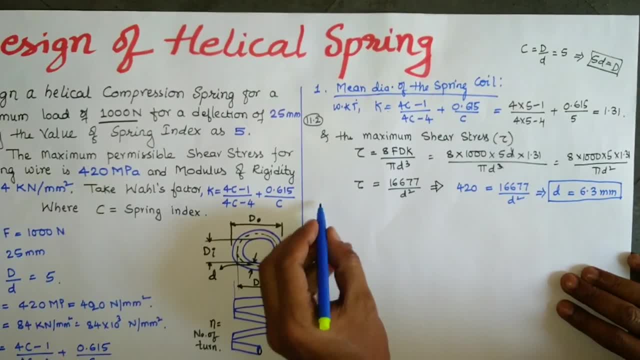 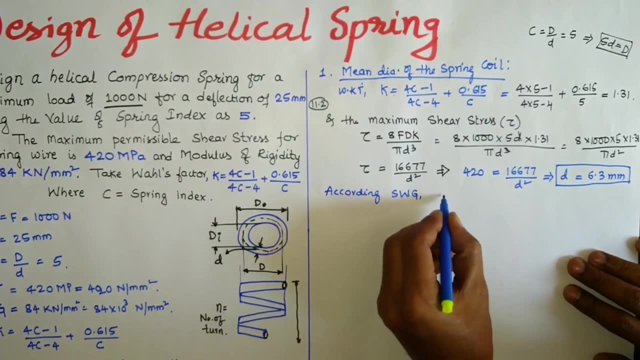 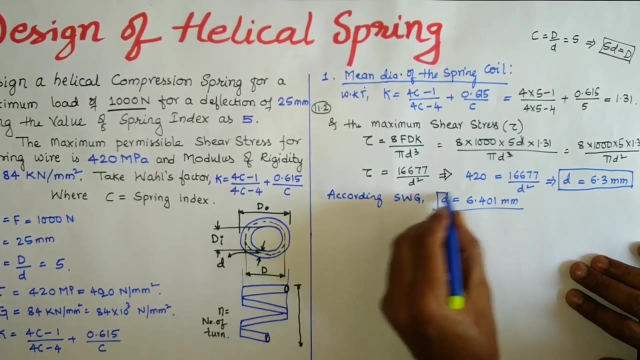 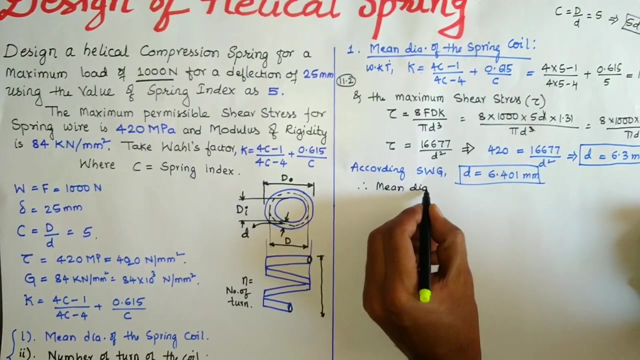 Okay, so 6.401 is the standard value. so now, according to standard wire gauge, the diameter of the coil is 6.401 mm, to be considered in the design. therefore, the mean diameter of the string wire is 6.401 mm. 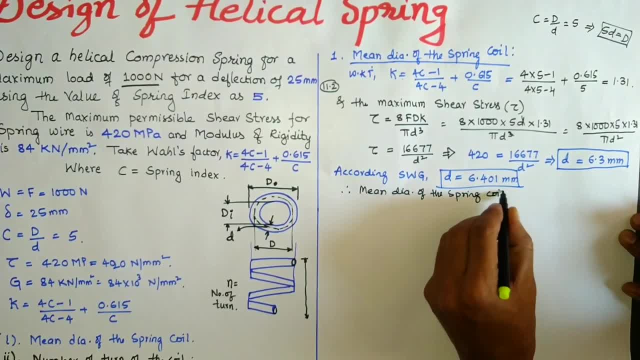 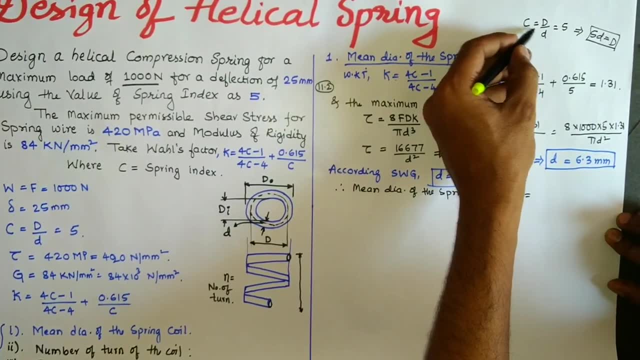 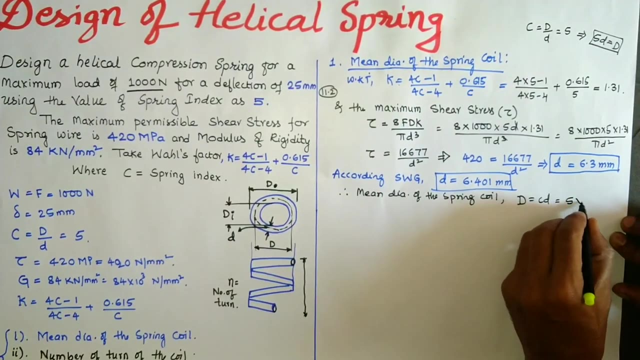 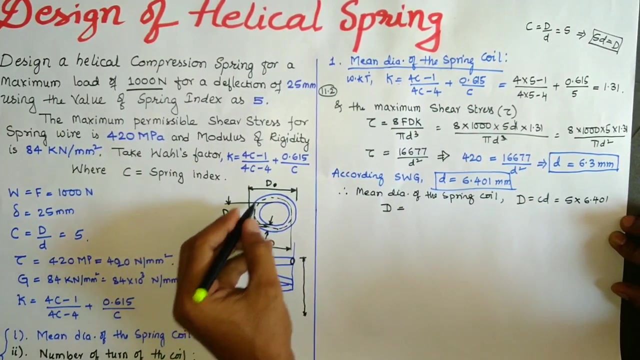 Therefore the mean diameter of the spring wire gauge is 6.401 mm. coil that is. d is equal to. so according to this equation, so d is equal to c into d. so mean diameter we are calculating. so c value is 5 and d value is 6.401. so we got mean diameter. so this: 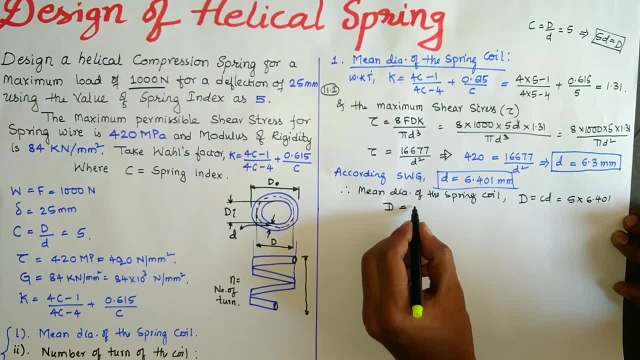 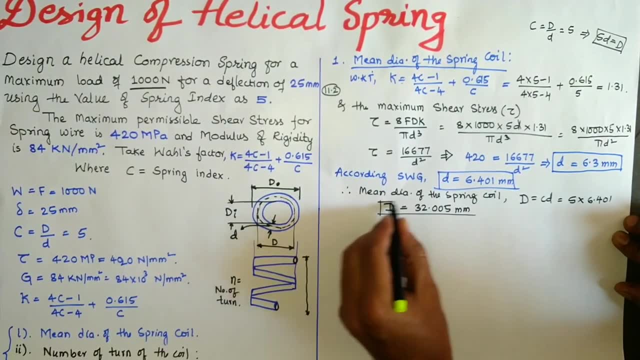 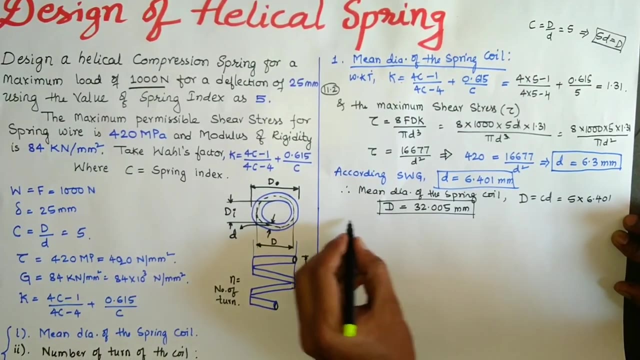 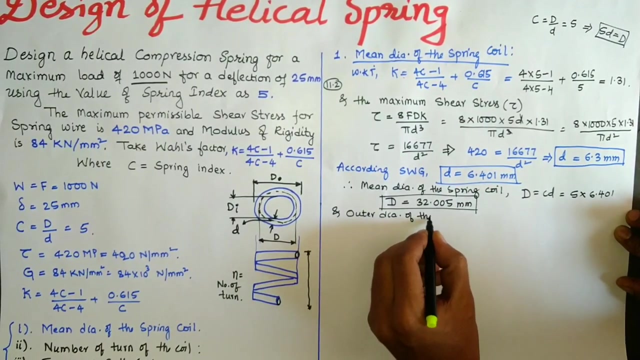 mean diameter we have obtained. so that is that value- is 32.005 millimeter. so once we calculated the mean diameter, then we will calculate the outer diameter also. so outer diameter we denoted with d naught and the outer diameter of the spring coil. so 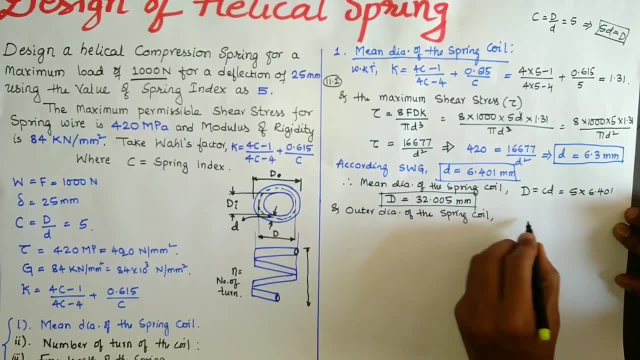 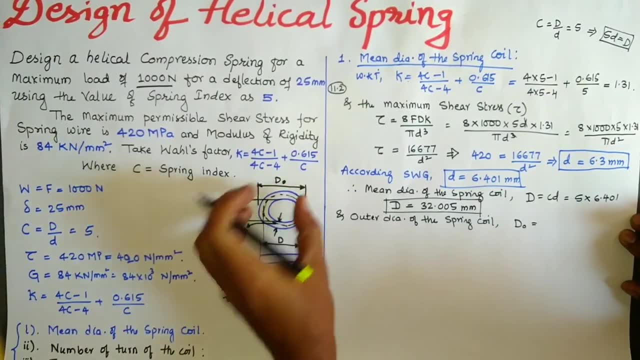 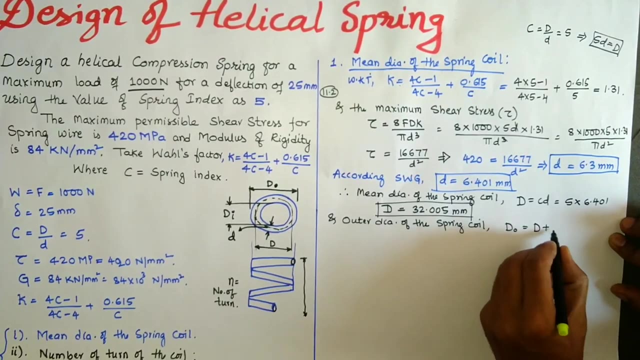 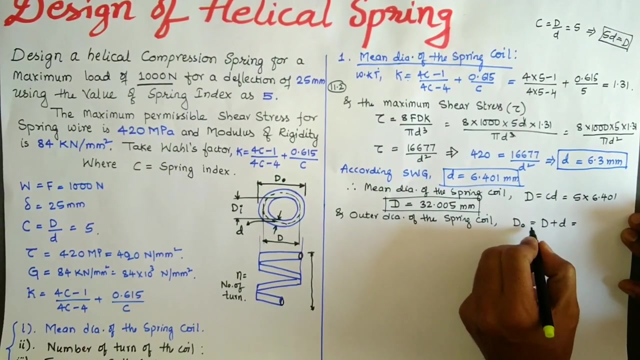 so. so so outer diameter of the spring coil, that equation. so d naught is equal to so for d naught it will be mean diameter plus diameter of the wire. so mean diameter plus diameter of the wire is equal to the outer diameter. so mean diameter outer for outer diameter, the value of mean. 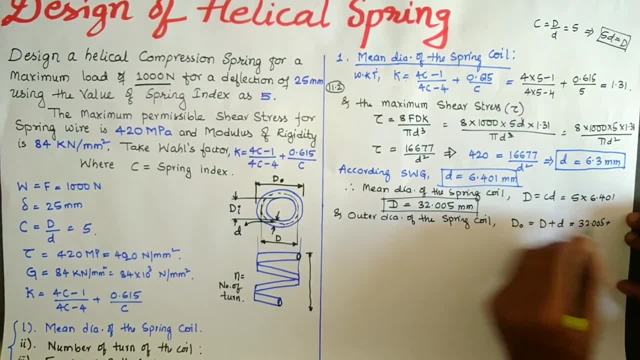 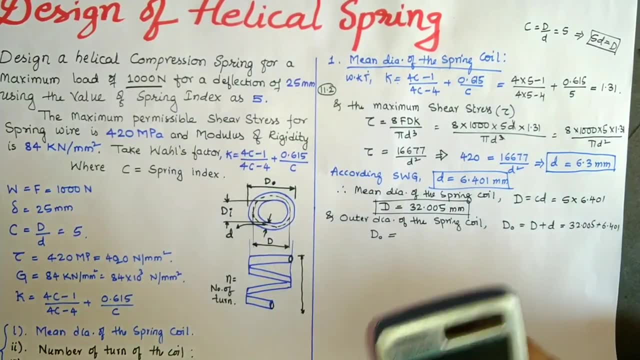 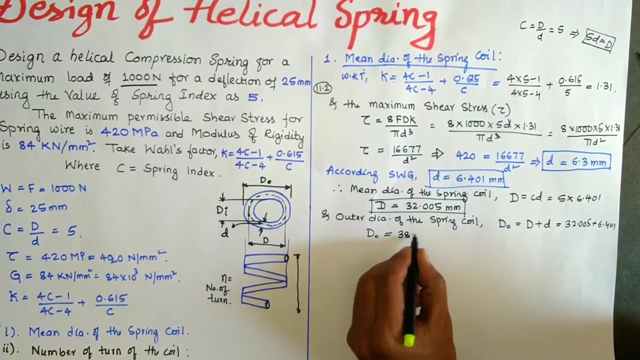 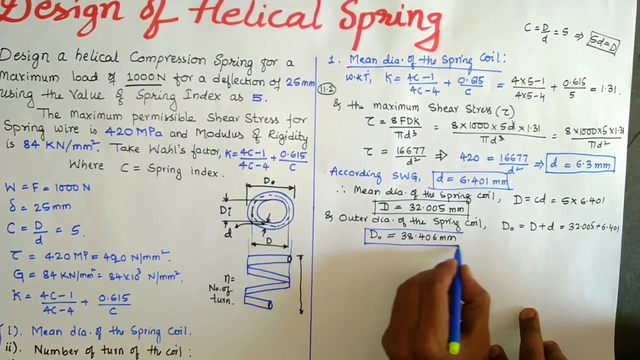 diameter is 32.005 plus 6.401, so so d naught is equal to, so the value is 38.406 millimeter is the obtained answer. so now, in the first step, we have completed mean diameter of this spring coil, where we have. 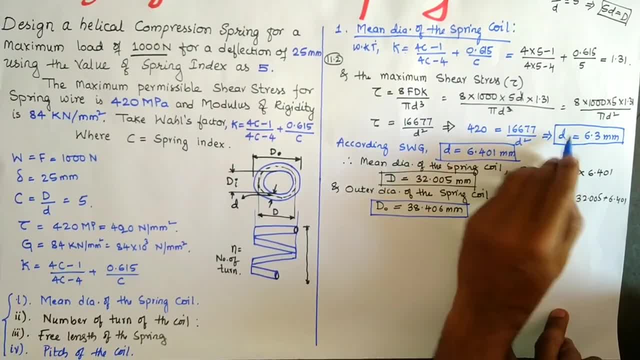 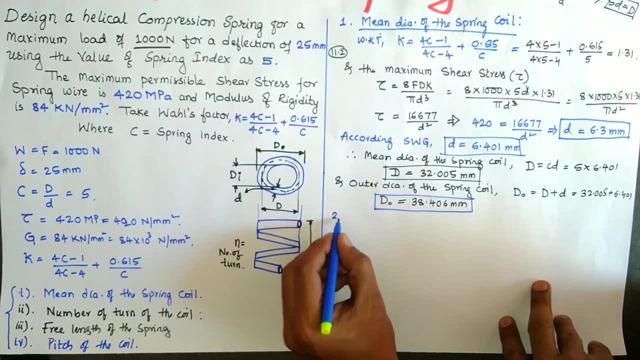 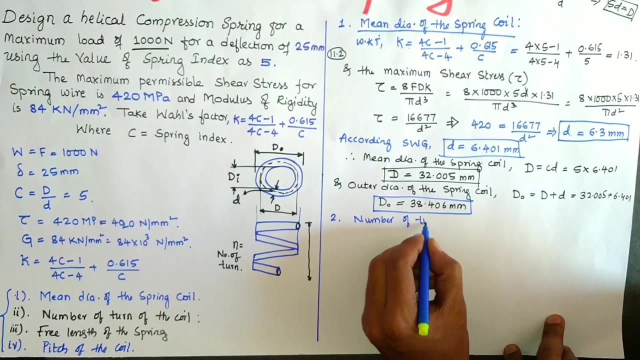 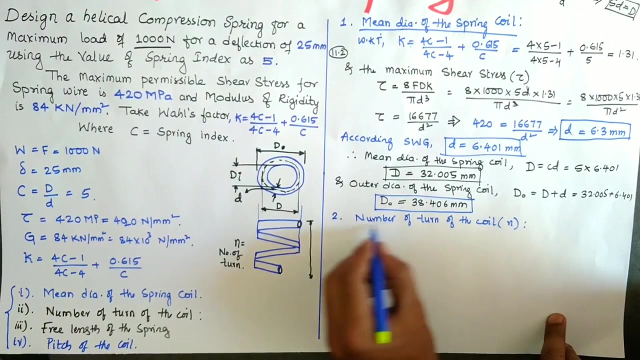 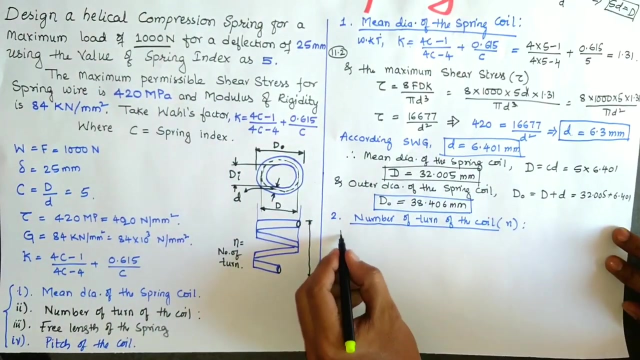 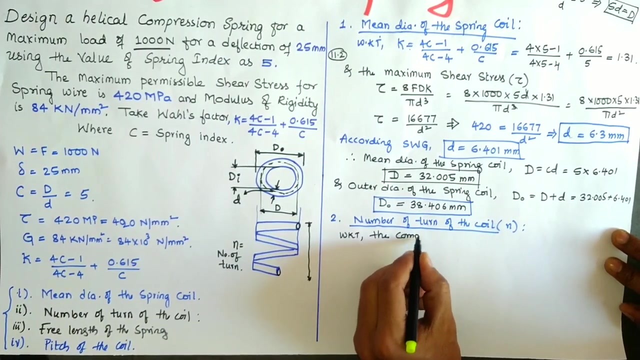 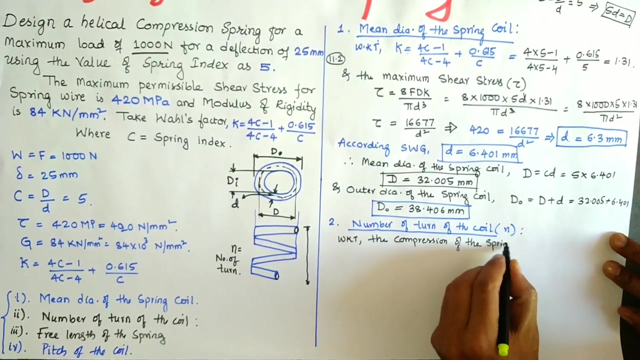 calculated the uh diameter of the wire and mean diameter and also outer diameter. The second step is to calculate the number of turns of the coil. that is small: n. So here, as we know that the compression of the spring, that is, delta, is equal to, so compression of the spring. So from the design data handbook we have, 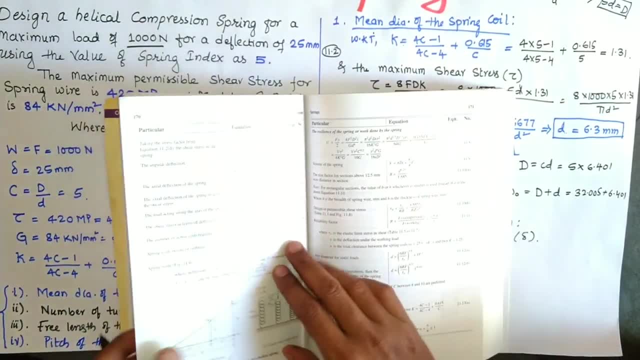 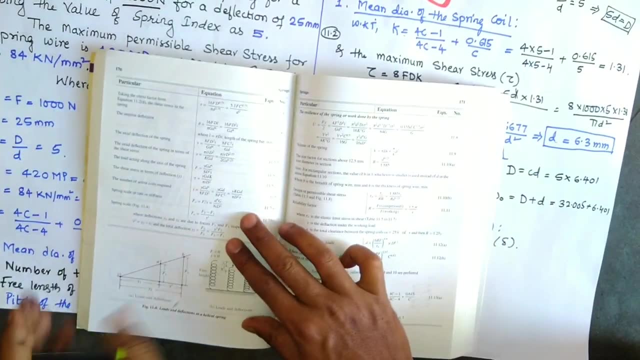 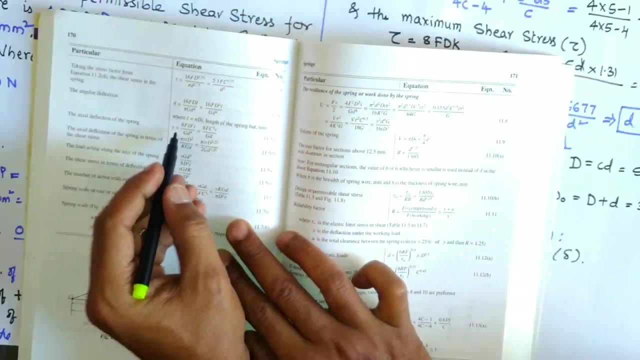 to find out what is the compression of the spring So delta. so here in the page number 178 from the design data handbook by Mahadevan. so where the deflection, axial deflection, of the spring so y, it is given, so y is also. 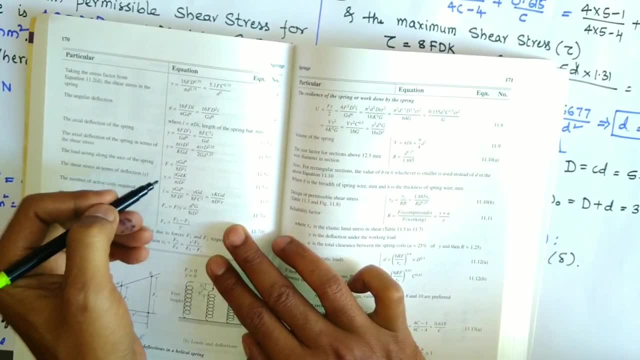 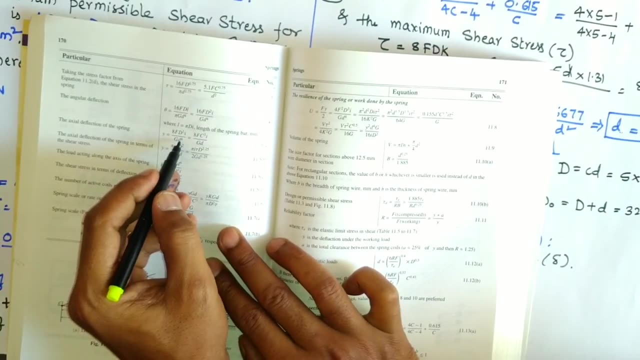 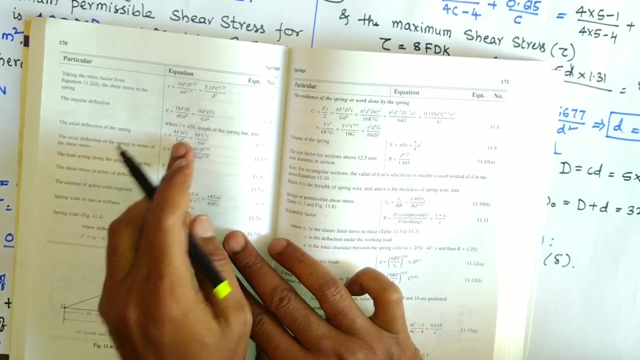 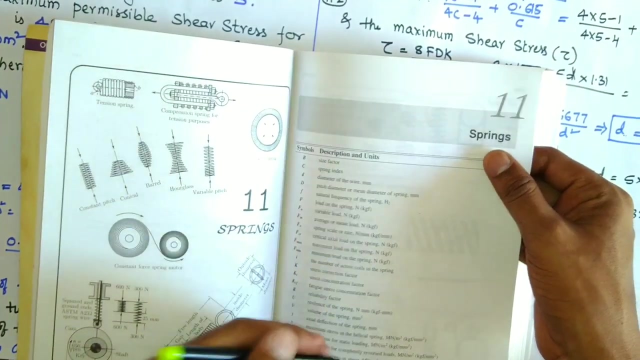 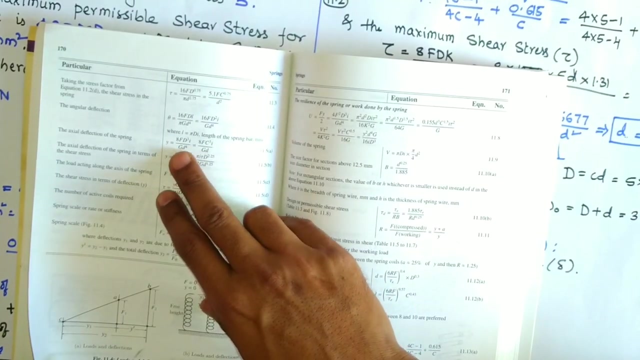 a deflection delta is equal to 8 f d cube i divided by gd power of 4.. So this equation is given where i, i- it is called as number of active coils in the spring. So we are saying n as i and f is the load, d is the mean diameter divided by g is the modulus. 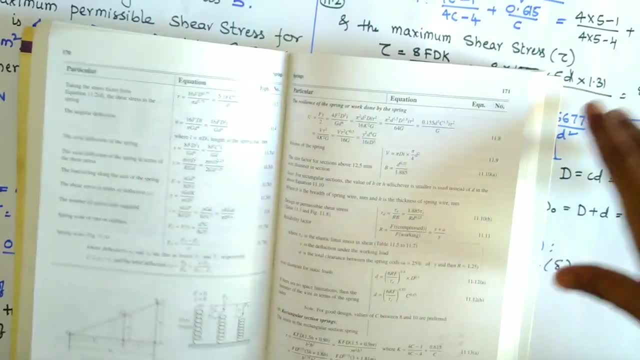 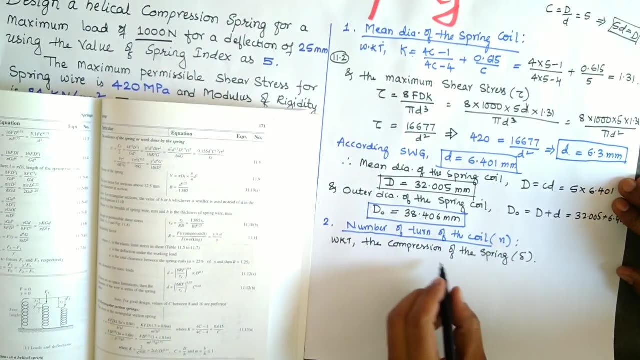 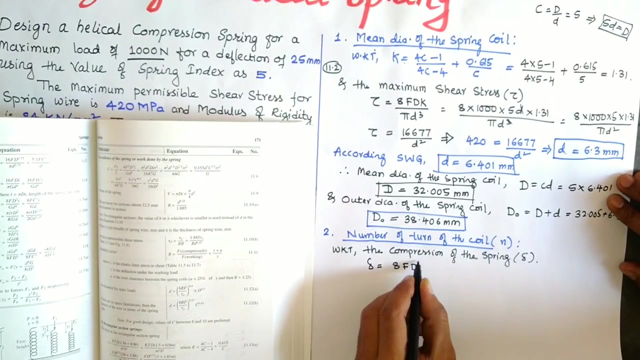 of rigidity divided into mean diameter of the coil. So we will write the equation. So we have to make a new equation. if we want to să, we will take the. if we want to have n add n, we will write this as d c power. of 4.. Now we have to do so. we can do amputation of the spring, which is called as n d, power of 4, so this is the distribution of the spring. So it is the distribution of the spring. that is 4, now it is not the, so it is the distribution of the spring like we have just. 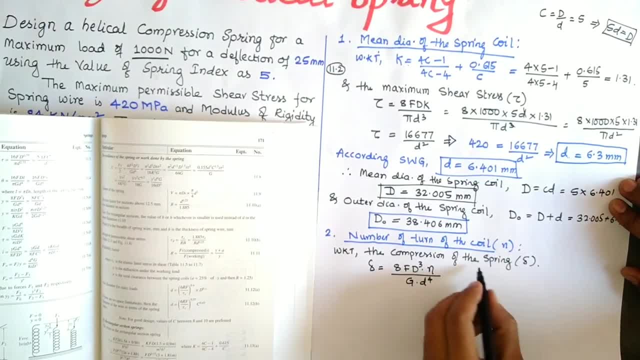 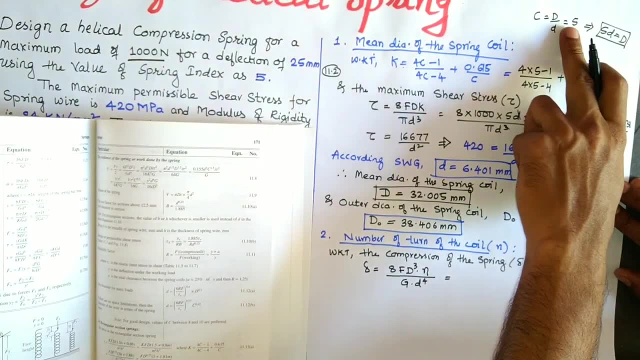 made. So n is the number of terms here. it is given as i in the design data handbook, gd power of 4.. So now we can make where from this data. if you substitute it f, 8f, it is equal to n. So from here we are getting that. so it is the number of terms here it. 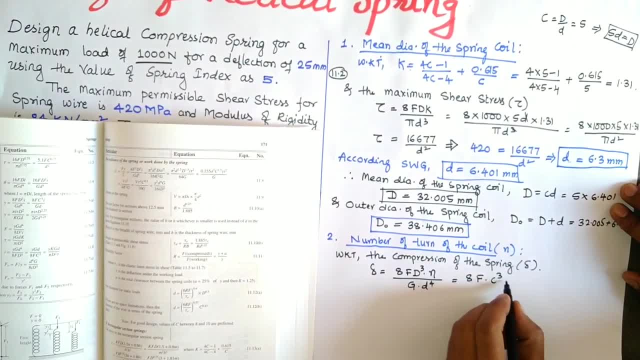 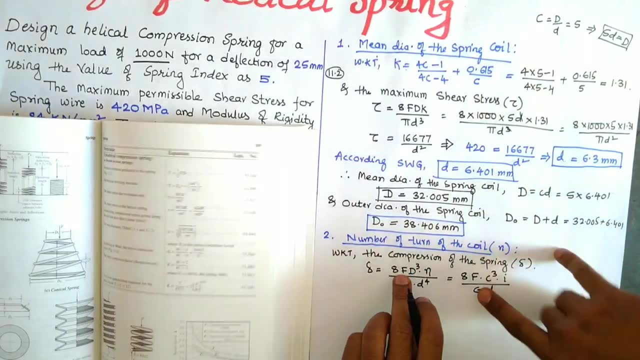 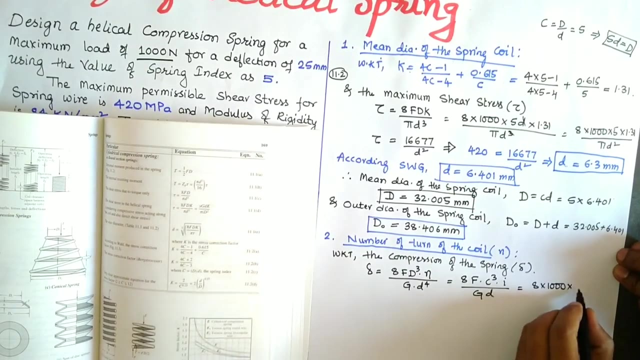 f, 8 f. so c cube into i divided by g, d we will get: if you substitute the value of d in the equation, we will obtain this one. so where 8 f is thousand into c value is 5 cube and i, i is nothing but n. 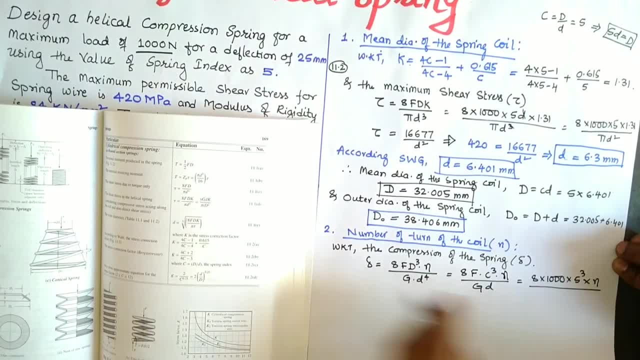 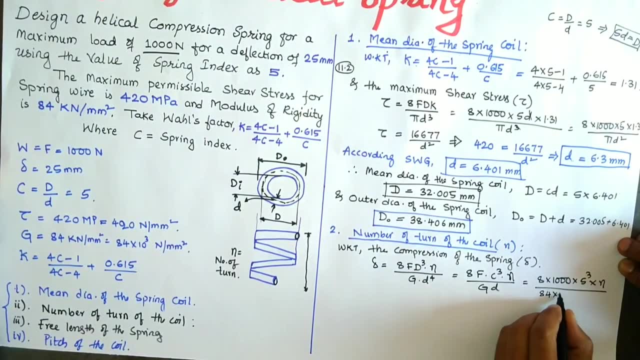 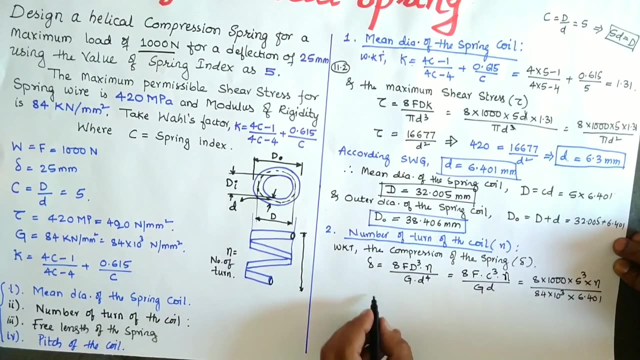 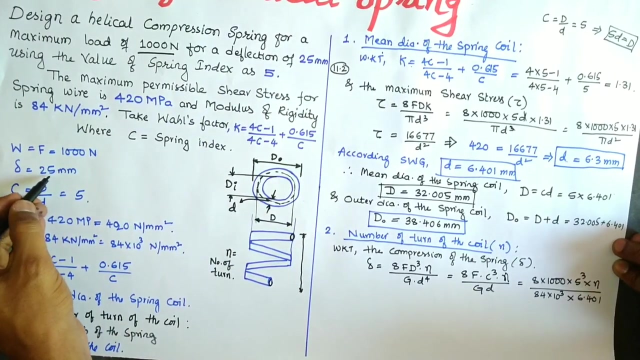 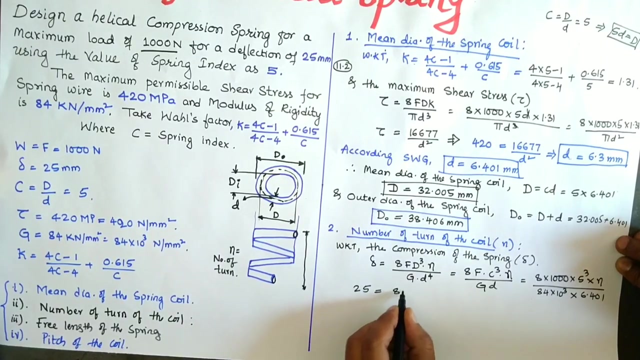 n will be the number of tons divided by g. modulus of rigidity is given as 84 into 10, power of 3 into d. d we got as 6.401. okay, and the delta? delta, it is also mentioned in the question. so that is 25, deflection is 25, so where 25 is equal to 8 into 1000, into 5 cube. 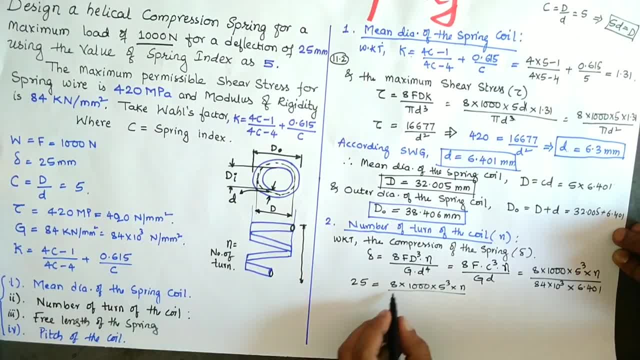 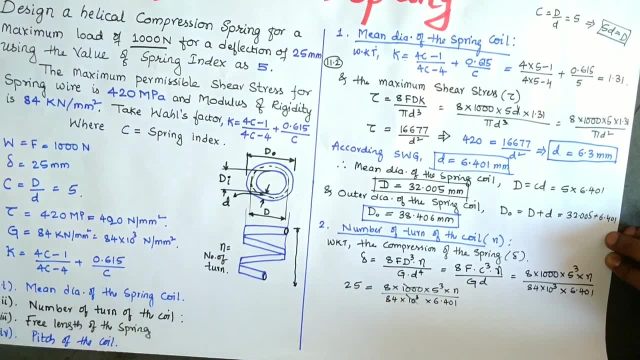 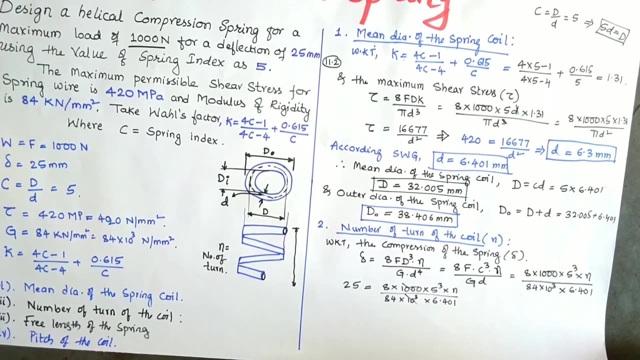 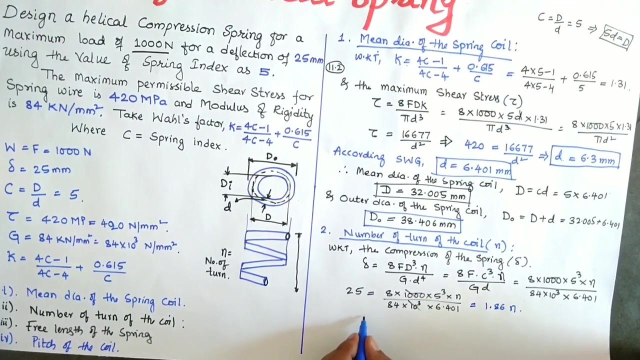 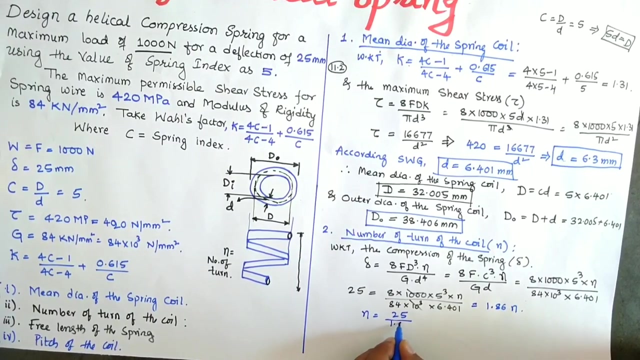 into n, divided by by 84 into 10. power of 3 into 6.401. so here it will get cancelled. so we will see what will be done. sir will get you. so I obtained one eight six into n, so where n is equal to 25 divided by one point. eight six, so 25 divided by one point. 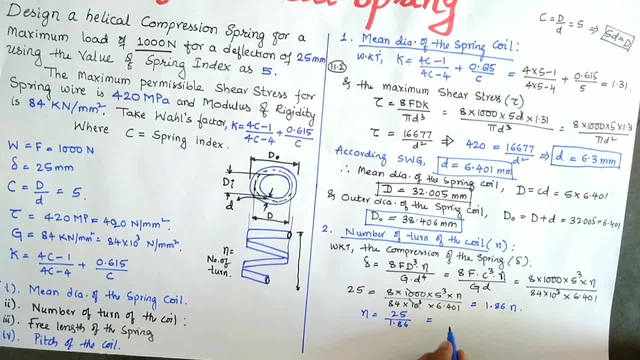 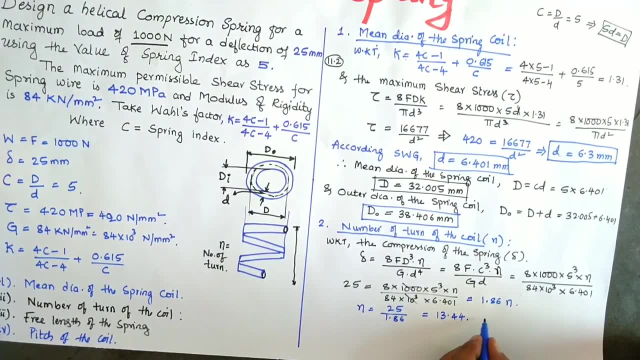 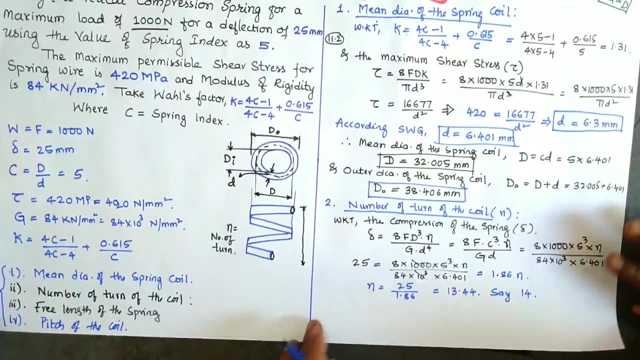 eight six. so 25 divided by one point eight six. so 25 divided by one point eight six is equal to thirteen point four, four. okay. so with the rounded value we'll say 14 is the number of tons in the spring. then the last one free length.